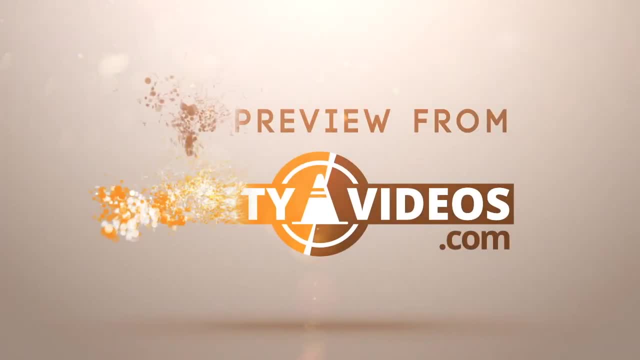 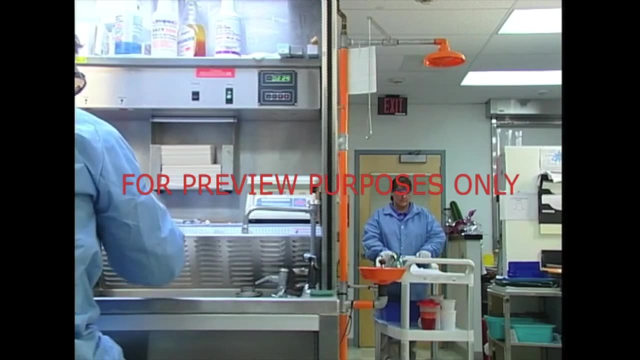 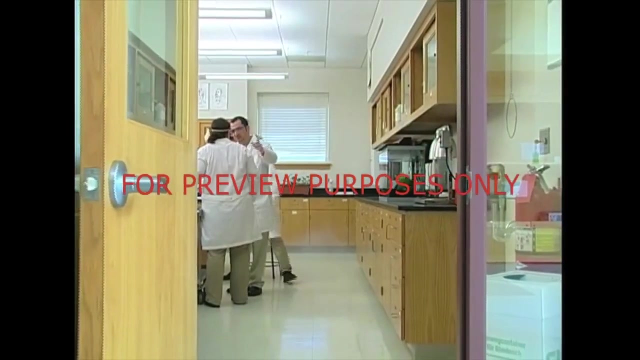 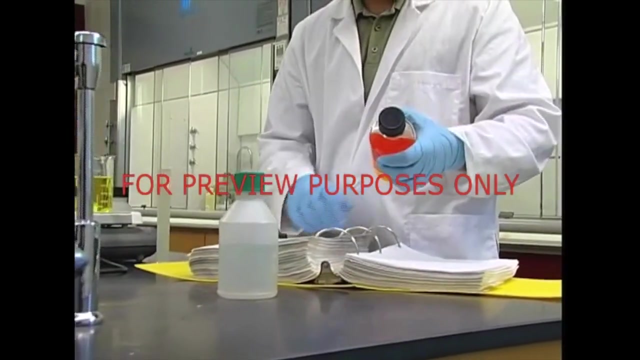 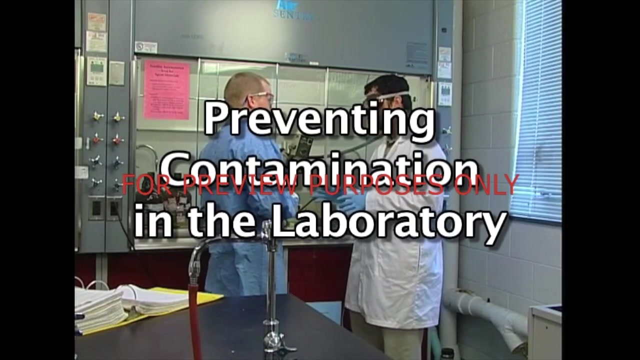 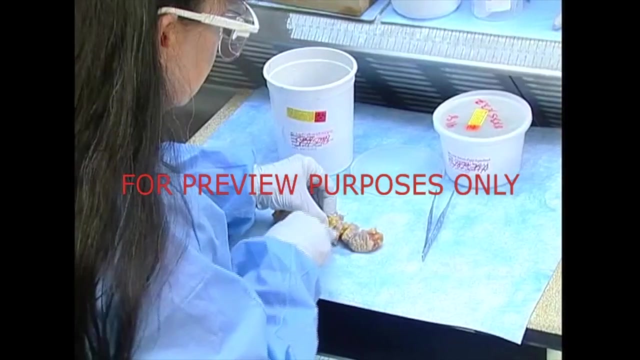 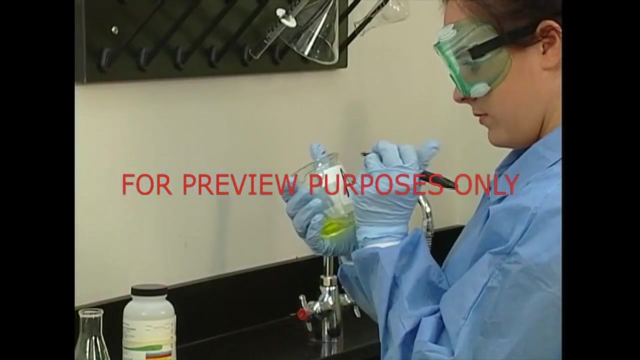 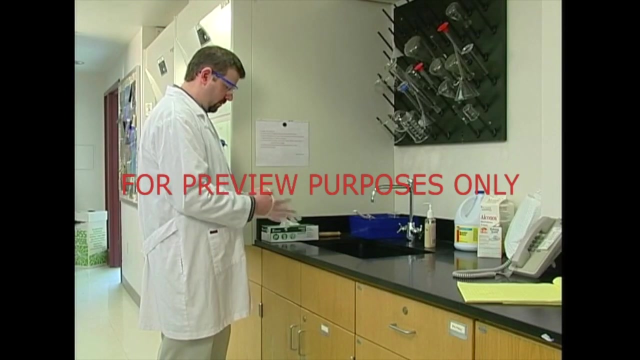 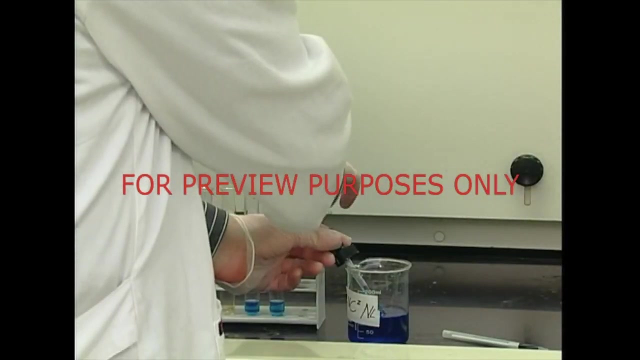 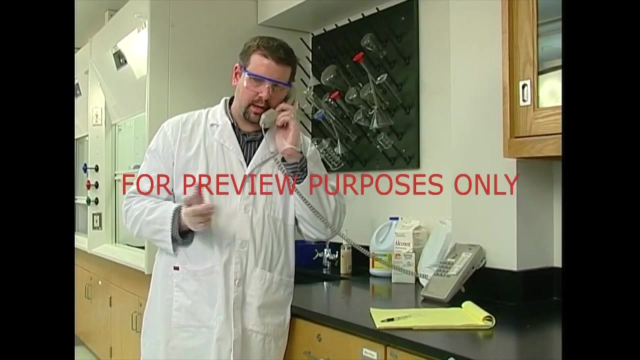 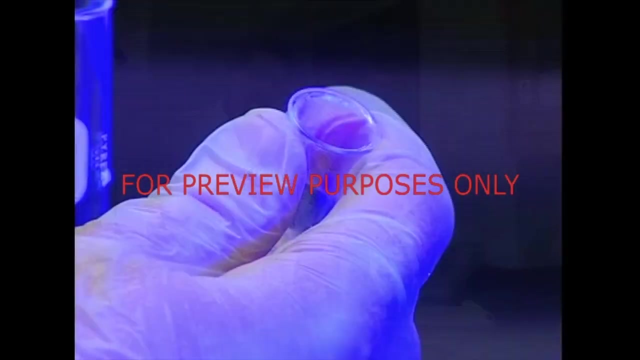 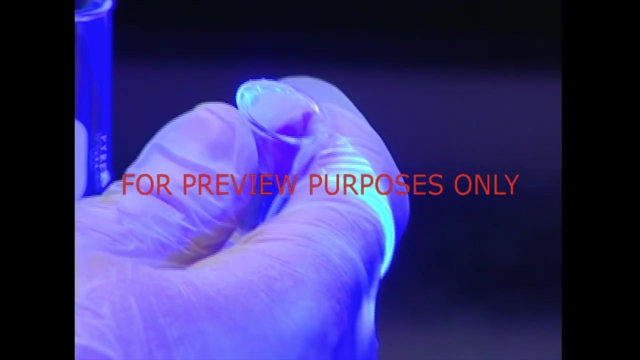 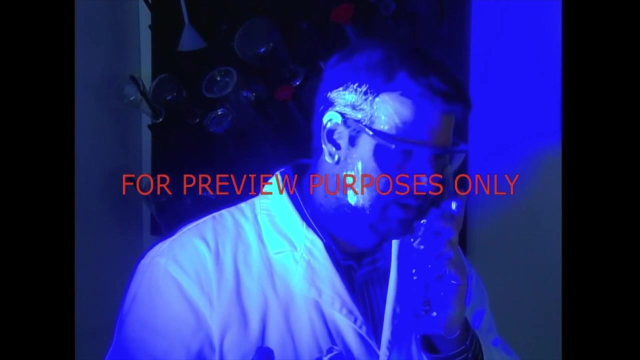 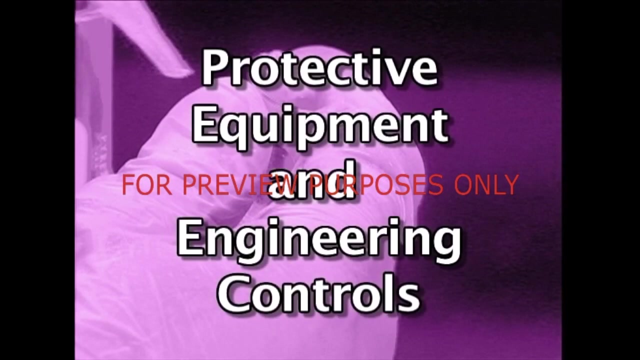 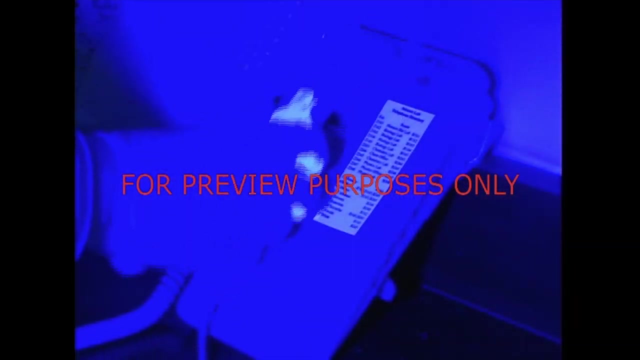 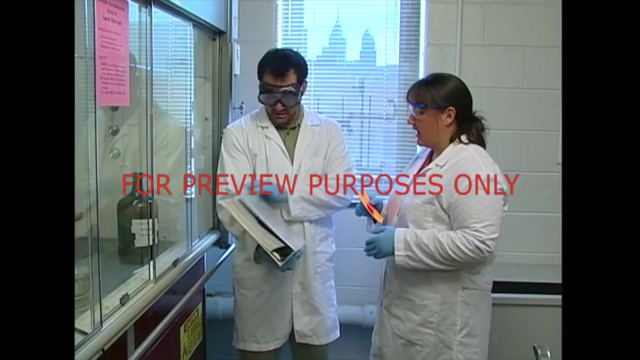 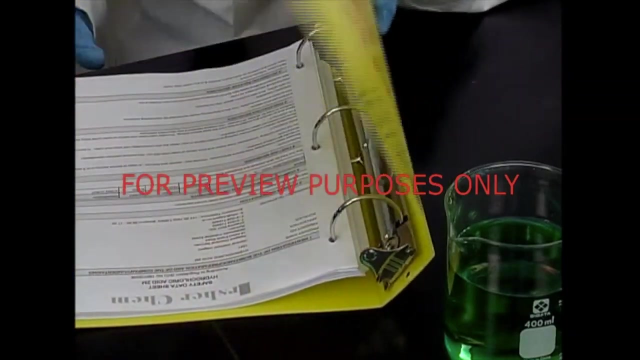 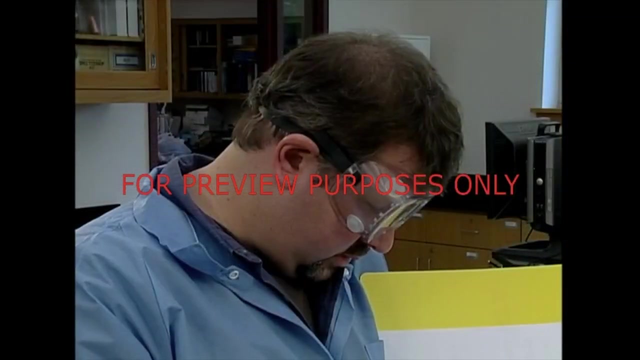 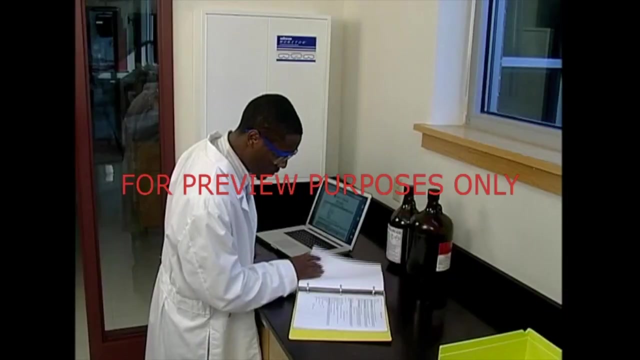 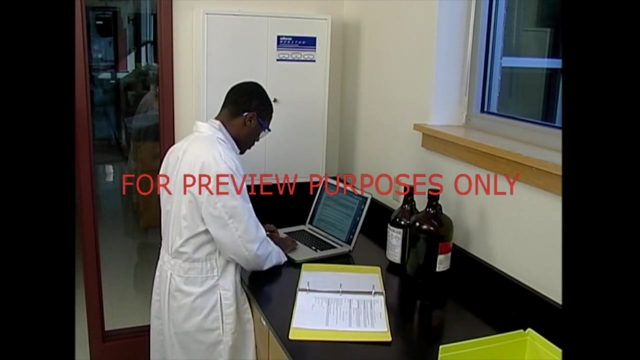 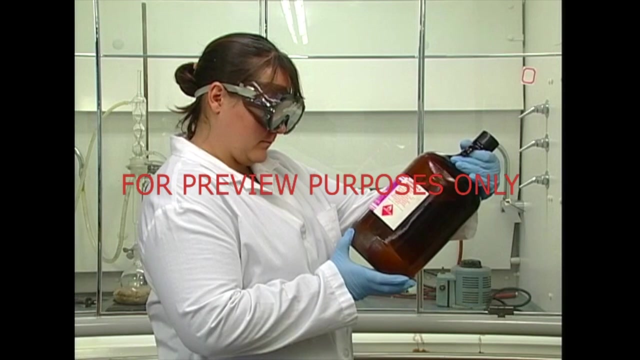 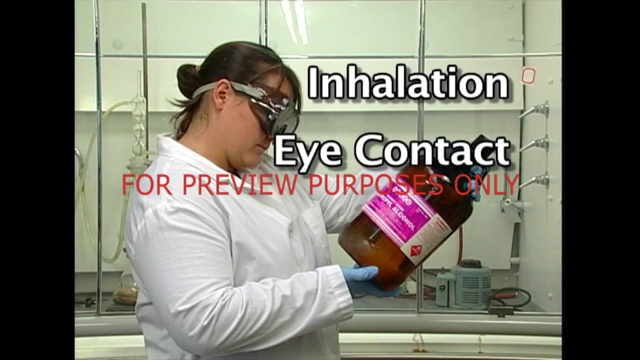 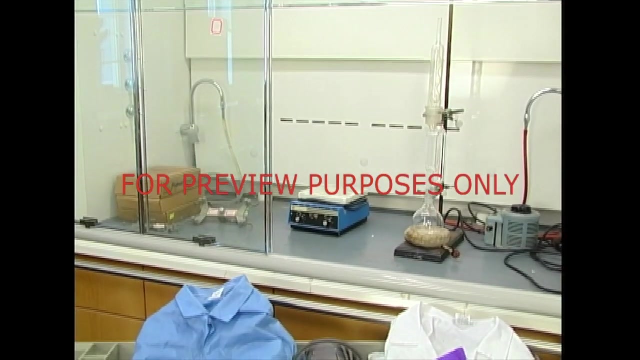 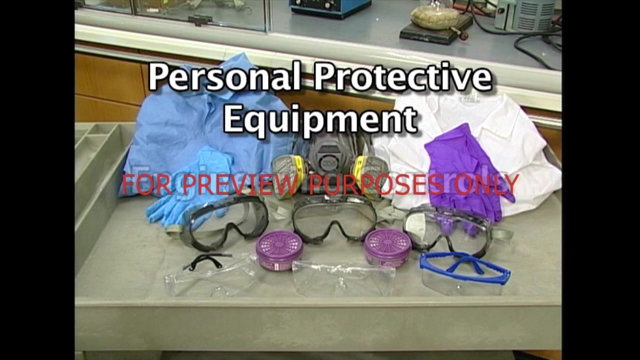 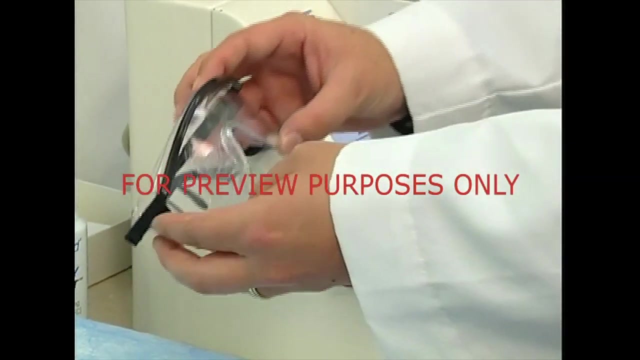 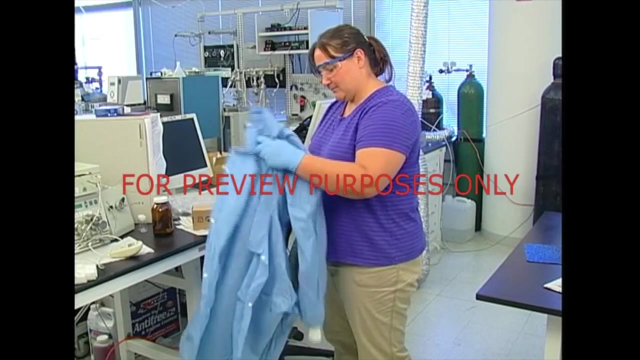 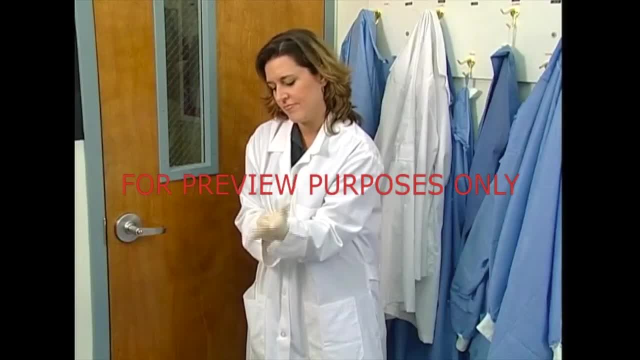 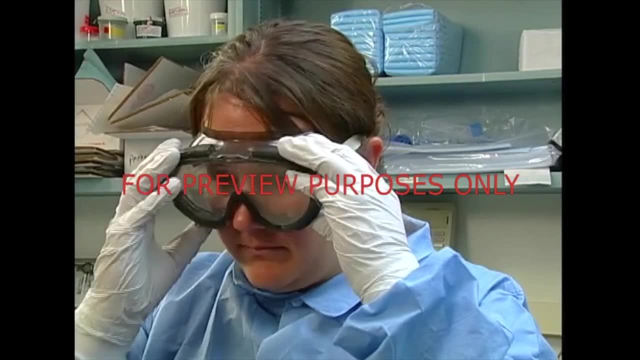 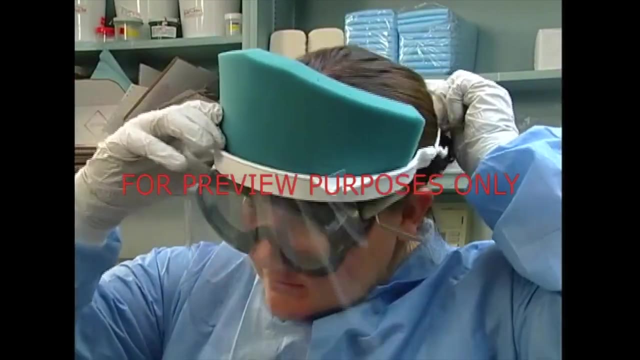 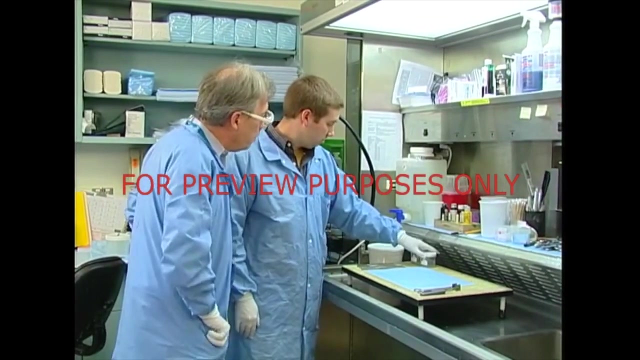 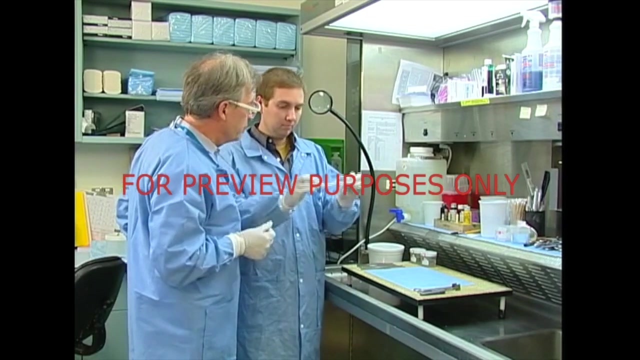 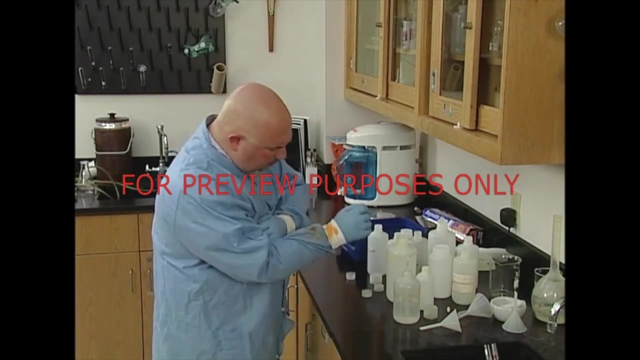 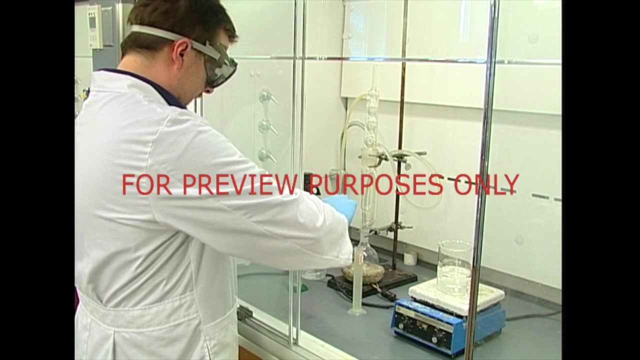 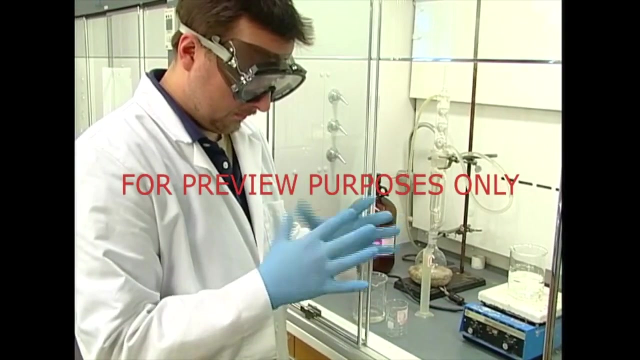 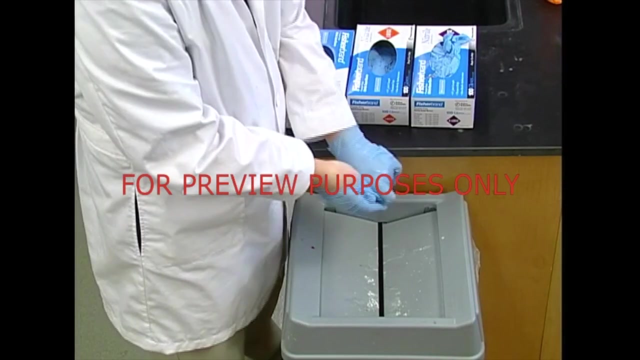 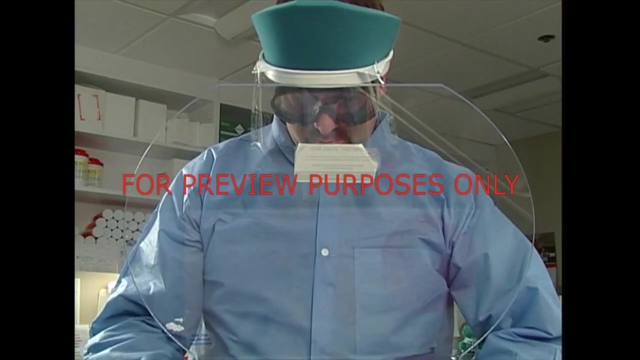 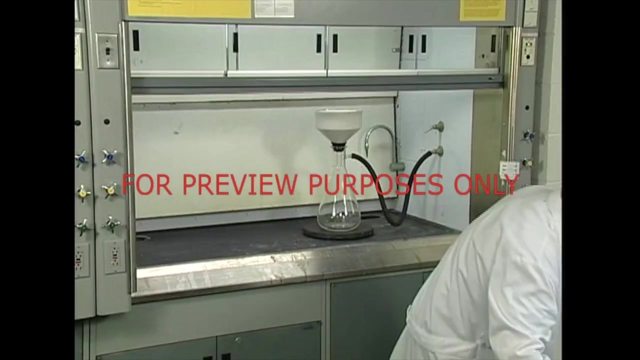 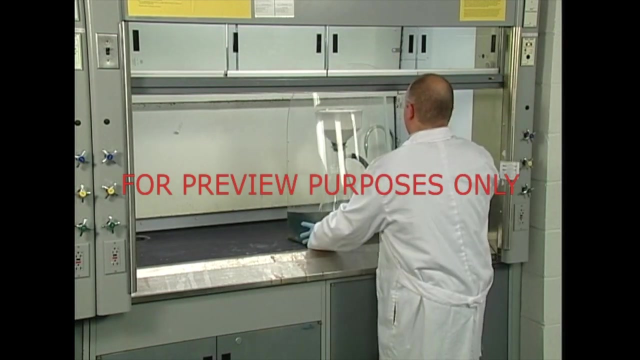 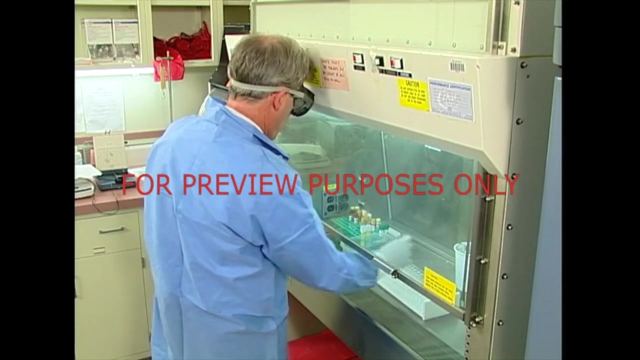 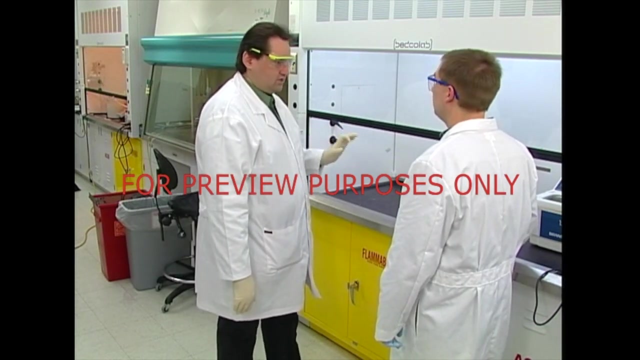 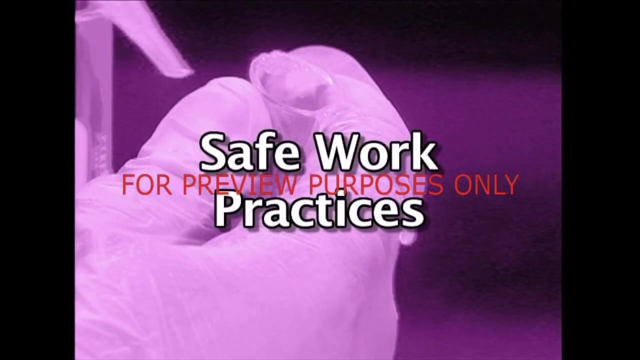 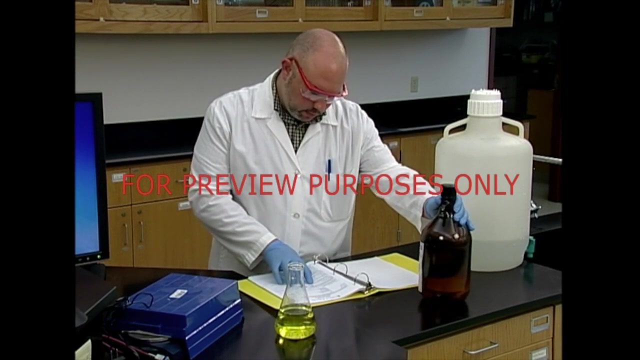 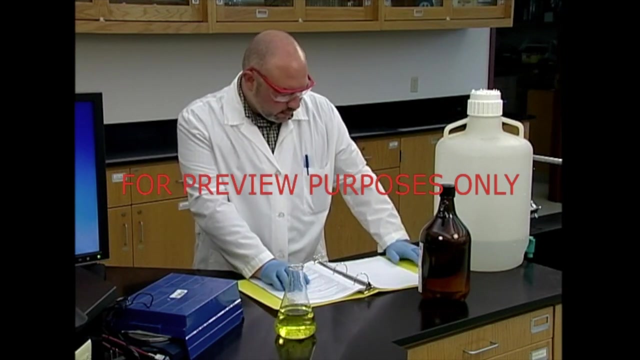 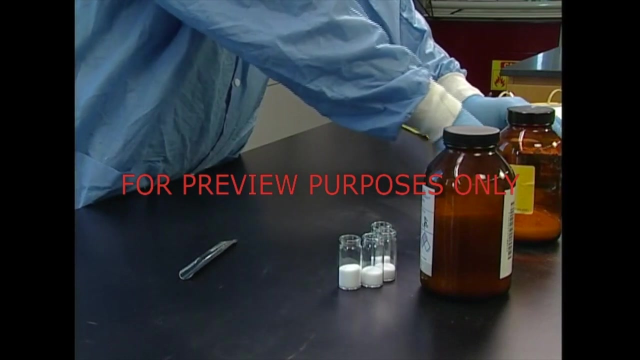 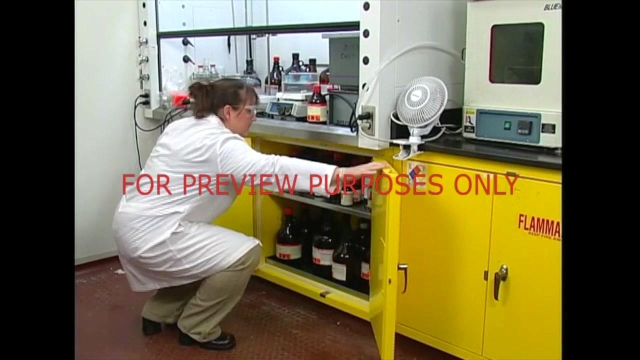 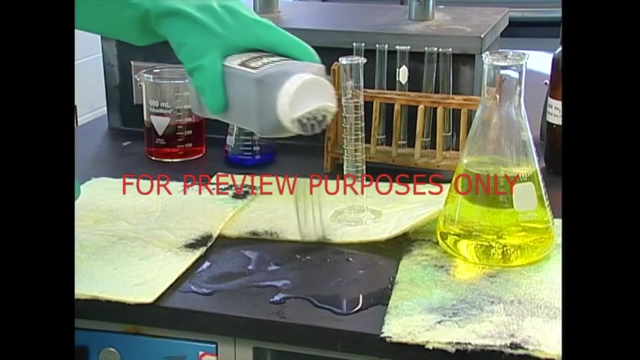 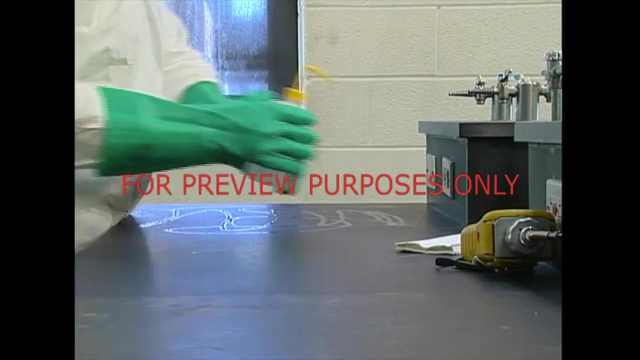 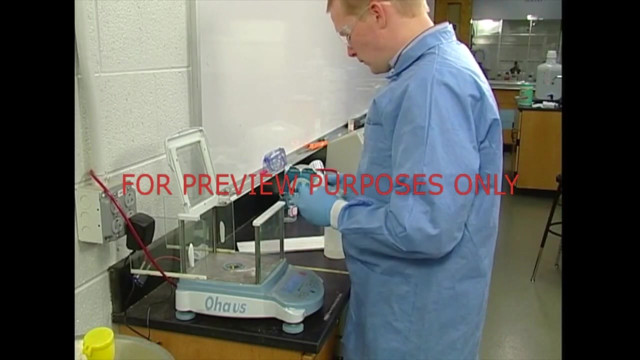 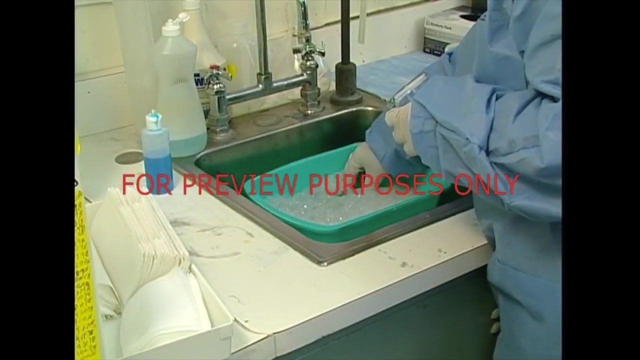 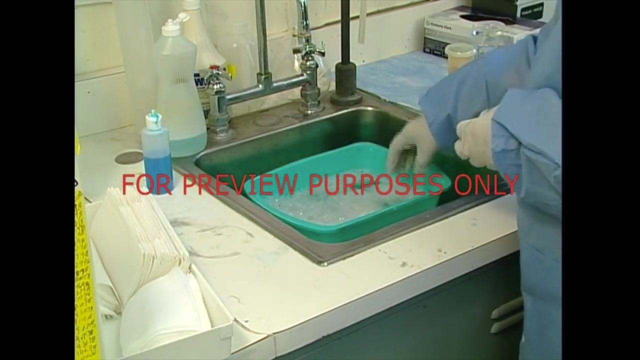 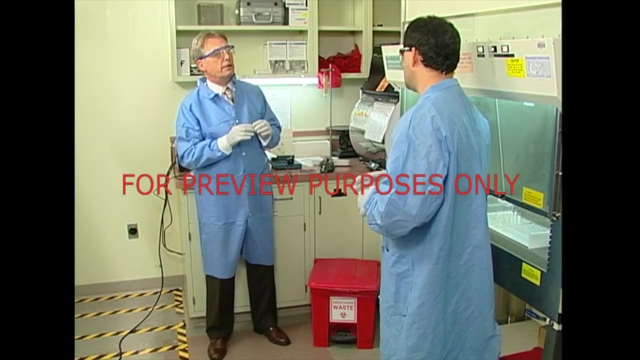 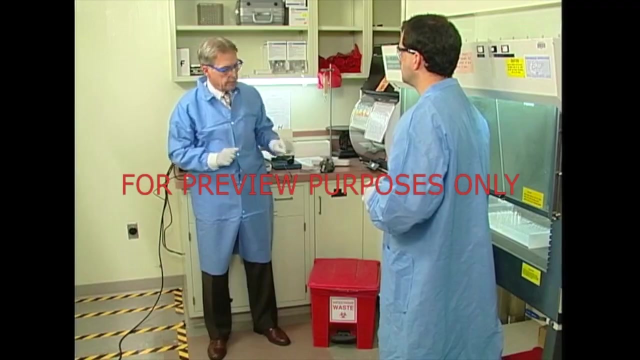 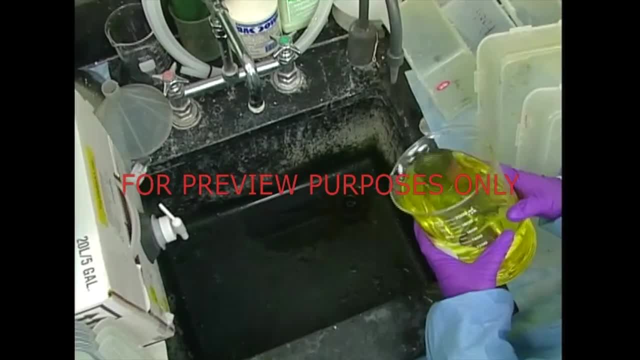 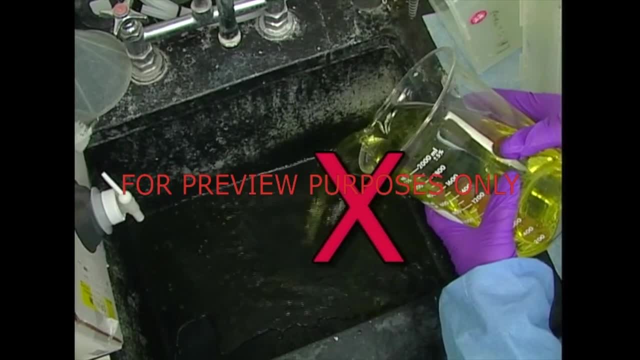 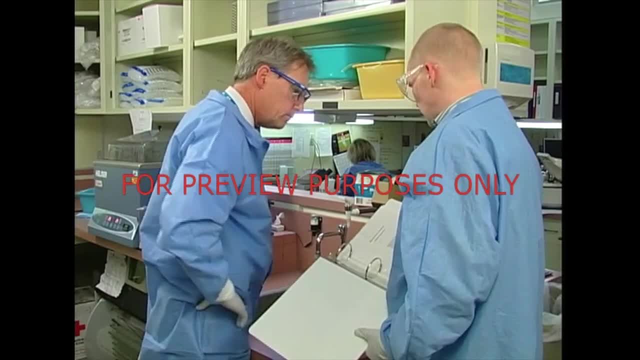 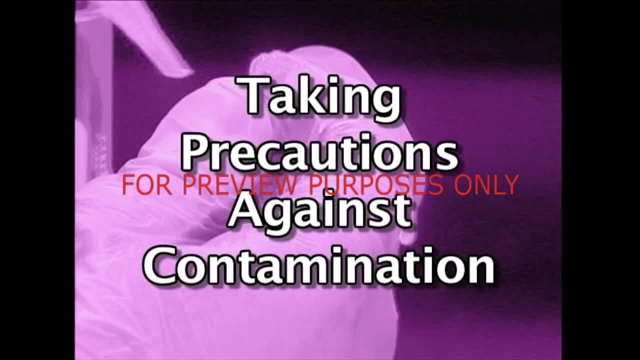 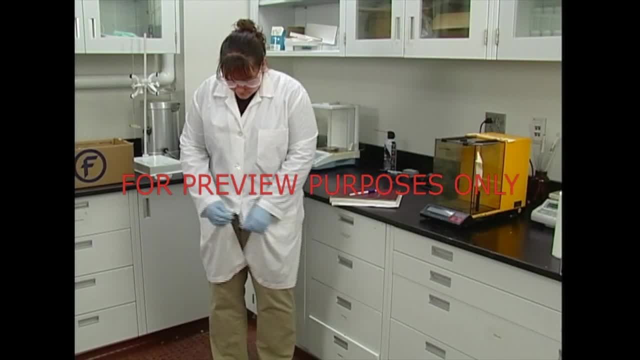 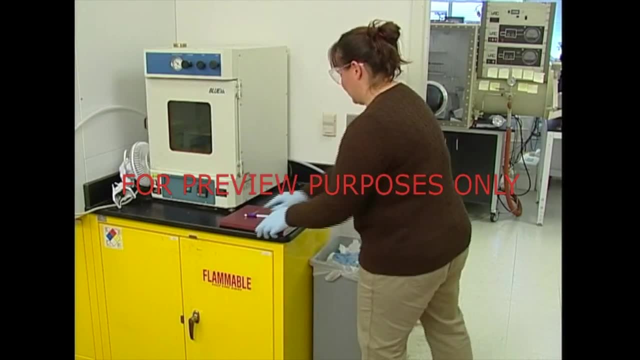 Transcription by ESO. translation by: —. Transcription by ESO translation by —. Another problem with contamination is its potential for personal transportation. When you're on a break off to lunch or on your way home, it can be easy to take a contaminant with you. 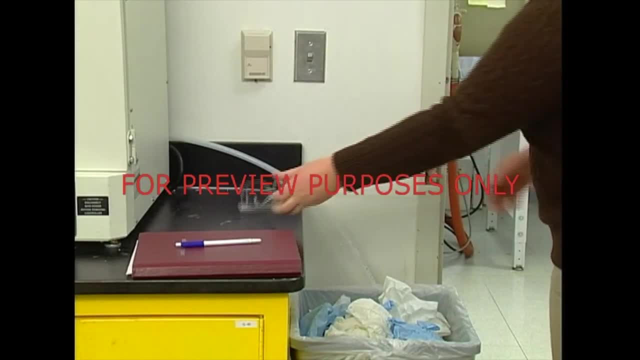 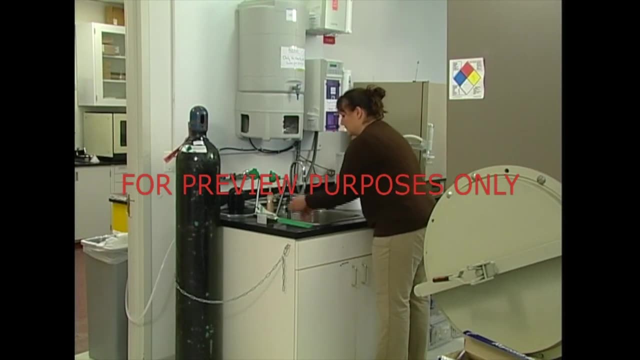 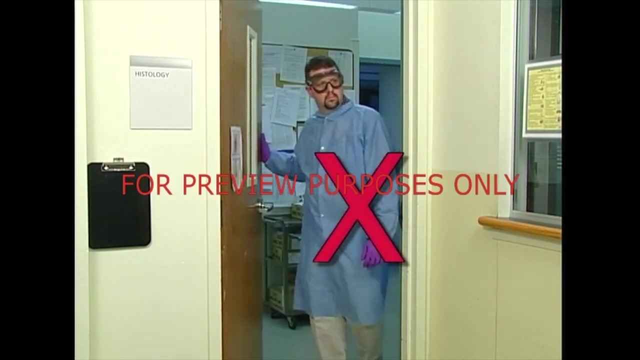 Leave notebooks, pencils and other supplies in the lab. Anything you use in your work should be thought of as being contaminated. Wash your hands thoroughly before leaving your work area. Never wear your PPE or lab coat outside the lab. That can cause real problems. 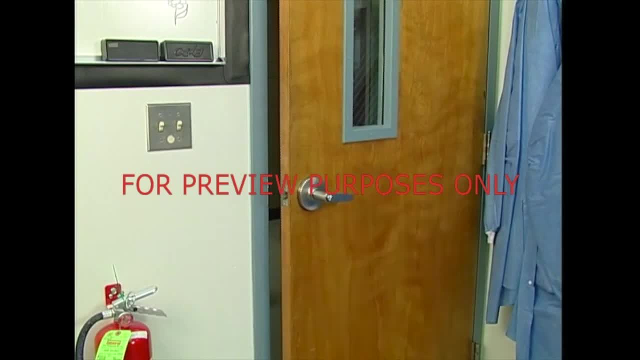 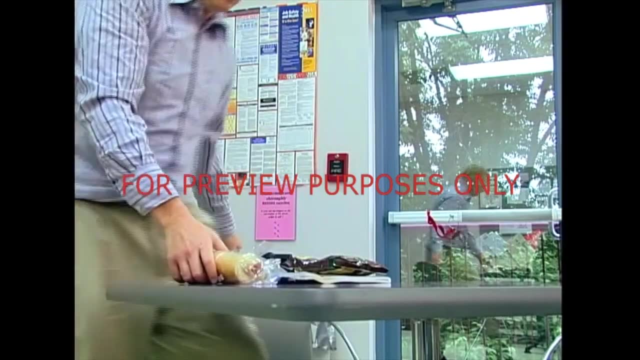 For instance, gloves can leave contaminants on doorknobs, which, in turn, can contaminate the next person coming through the door. Poor safety practices can also increase the risk of ingesting hazardous materials. Something as simple as taking your laptop and your laptop case with you. 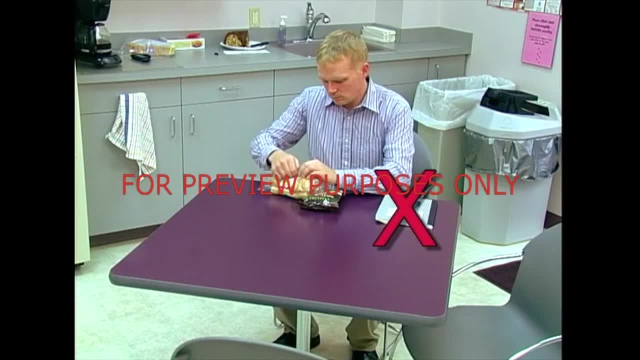 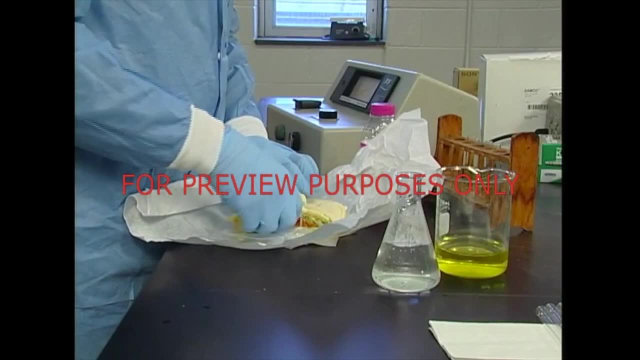 Or taking your lab notebook to lunch could lead to contaminating your sandwich. Of course, this type of problem can also occur inside the lab. Never bring food or drink into your lab area And don't wash your coffee cup or lunch dishes in the lab sink. 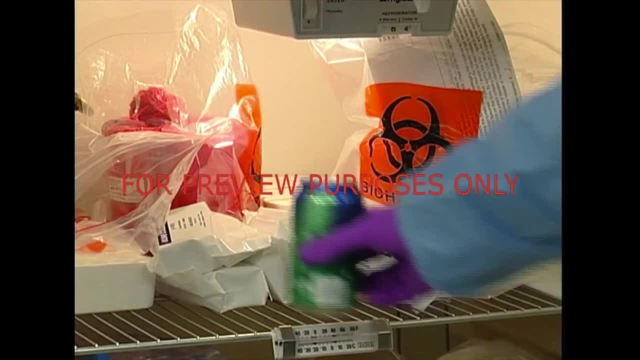 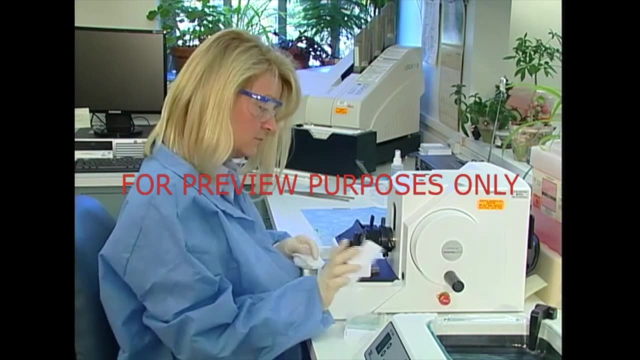 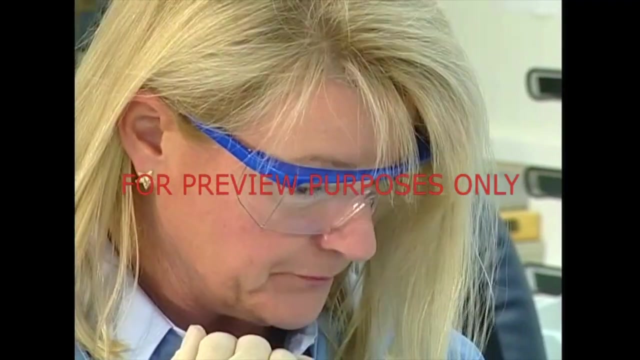 The rule of thumb for avoiding ingestion hazards is: never mix contaminants with uncontaminated objects or areas. You also need to remember that contaminants move easily from one place to another, So you should avoid nervous habits like rubbing your face or scratching your nose. They can bring hazards too close to your mouth. 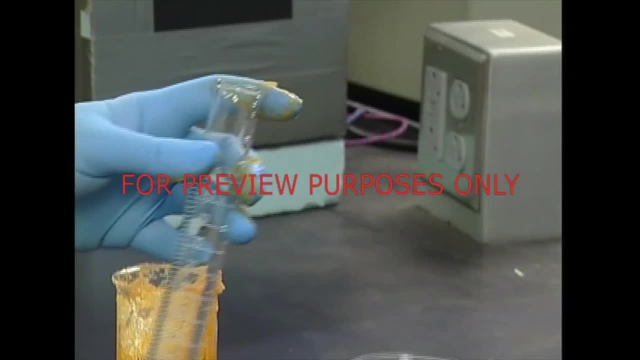 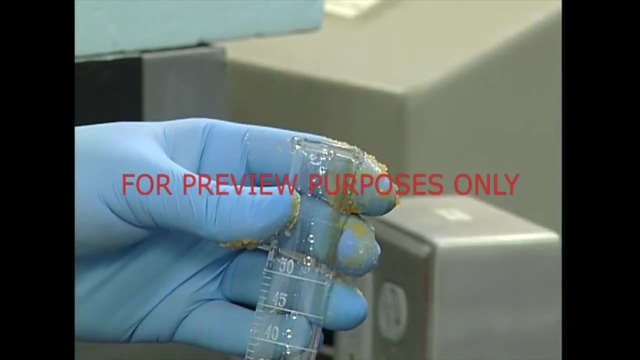 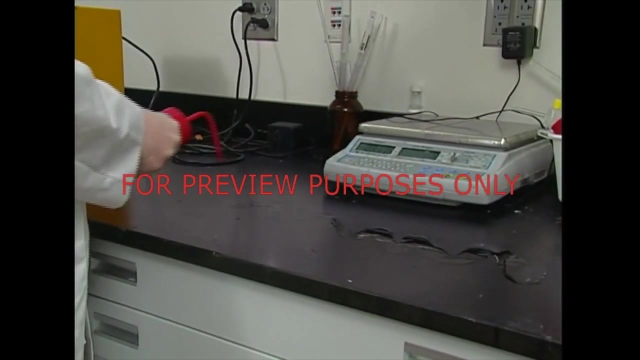 It's also important to protect the materials that you're working with from contamination. It's all too easy to contaminate a sample with a chemical unknown. that can result in a false reading. To prevent the contamination of samples and other materials, keep your work surfaces and equipment clean. 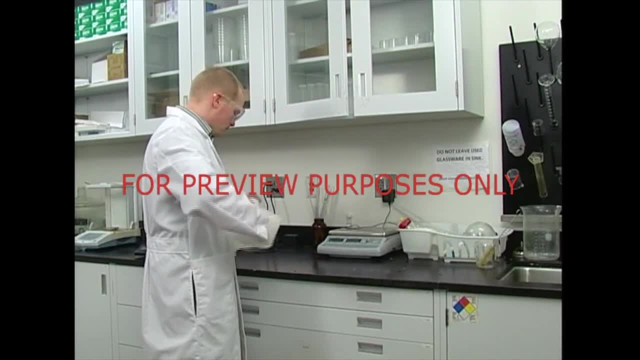 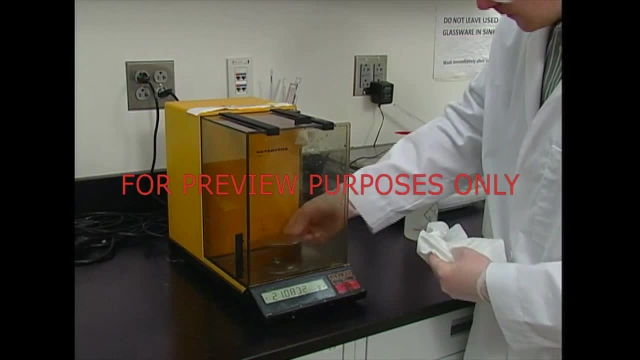 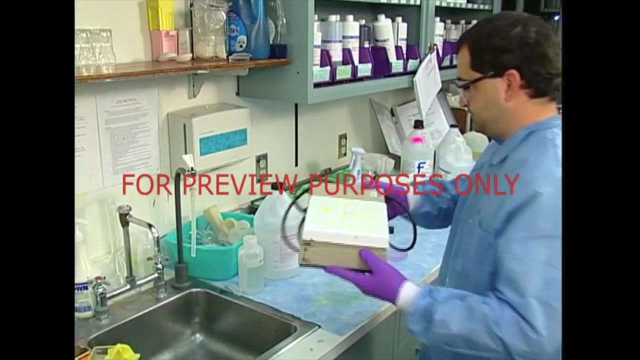 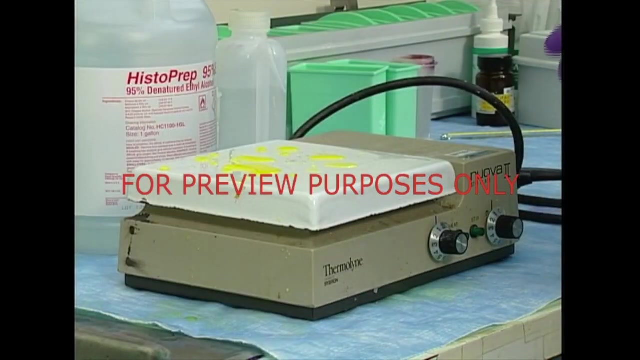 Check them before, during and after your work. Decontaminate all equipment after using it. Be thorough. Follow your lab's established cleaning procedures. Pay special attention to equipment that's shared with other workers. Hot plates and stirrers, for example, tend to collect chemical residues over time.